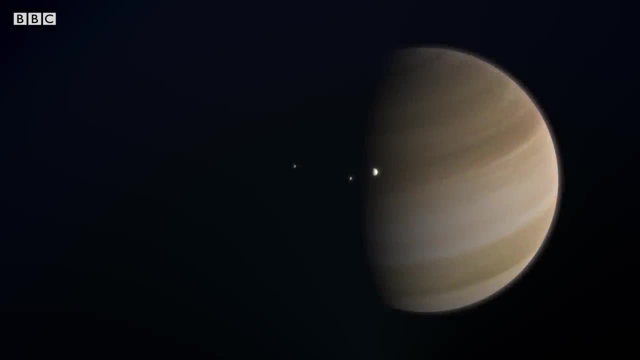 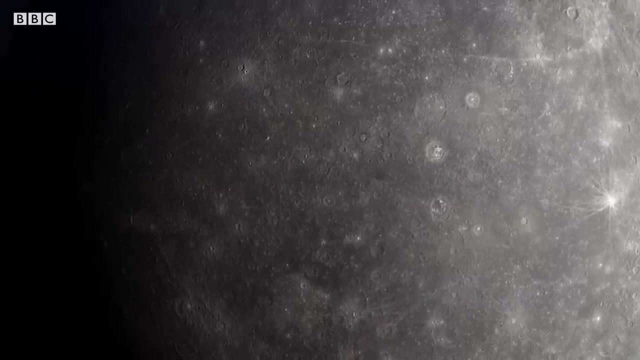 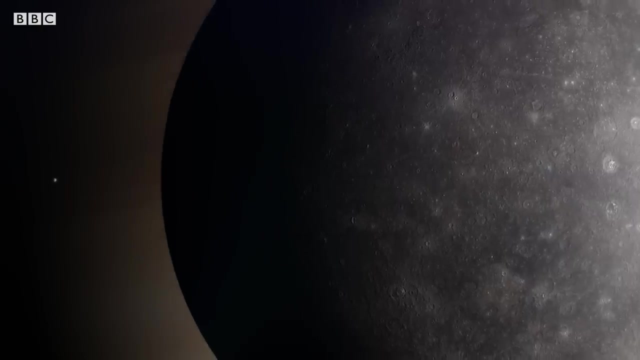 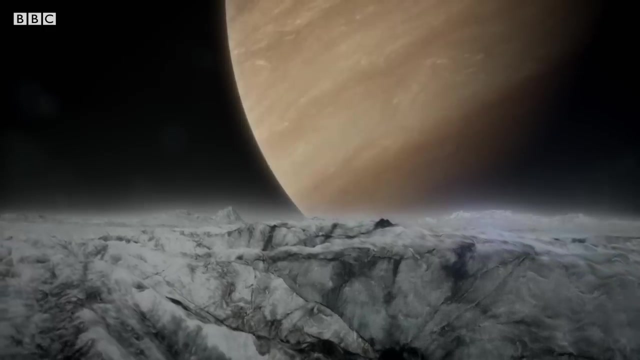 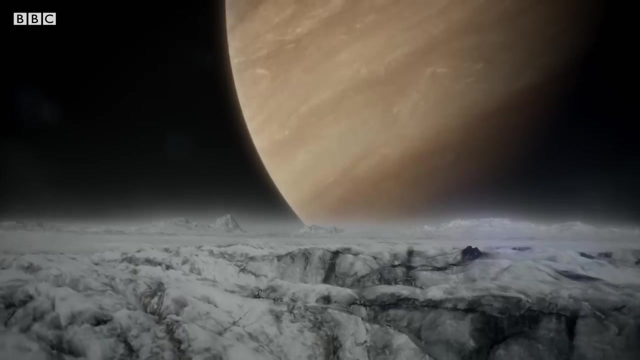 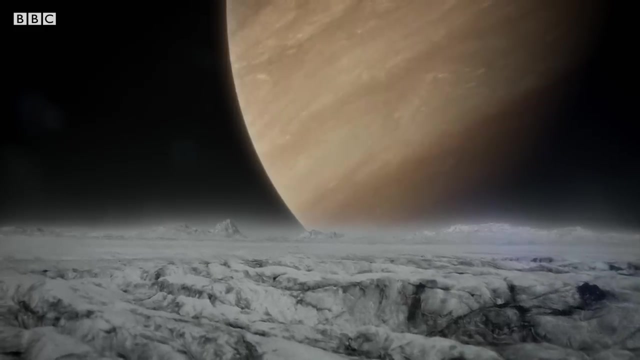 Millions of years ago. Saturn has an extra moon, Perhaps 400 kilometers across and formed almost entirely of ice. But this moon is doomed. It's orbiting just too close to resist the immense forces of Saturn's gravity. The rings probably formed from an object that got too close to Saturn. 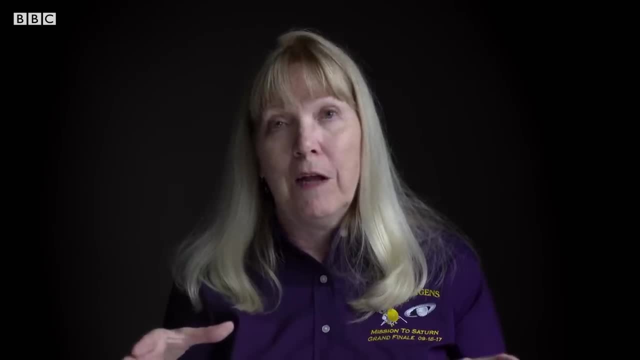 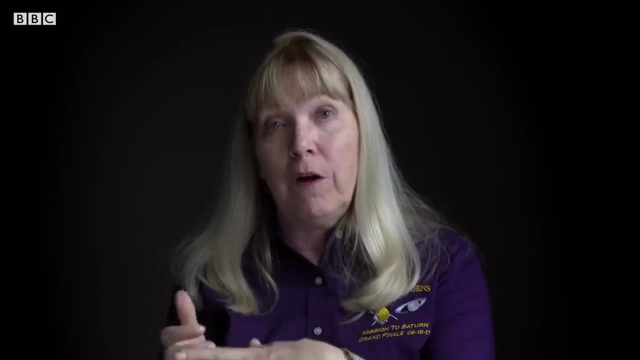 There's this invisible boundary around Saturn called the Roche limit, And that's the limit, depending on what you're made of, where Saturn's gravity is strong enough will actually pull you apart That the gravity on the side closer to Saturn is strong enough. that, compared to the gravity on the other side. that 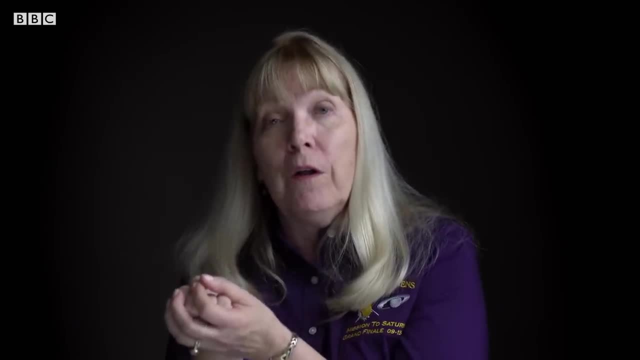 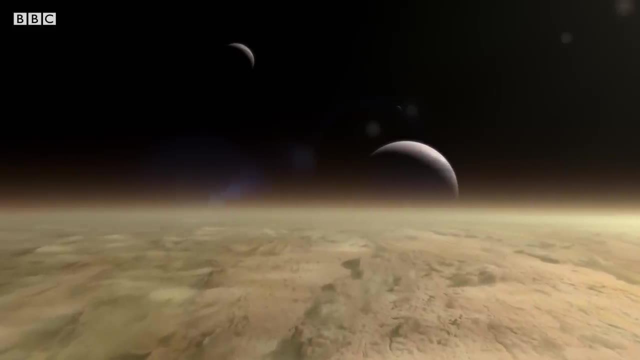 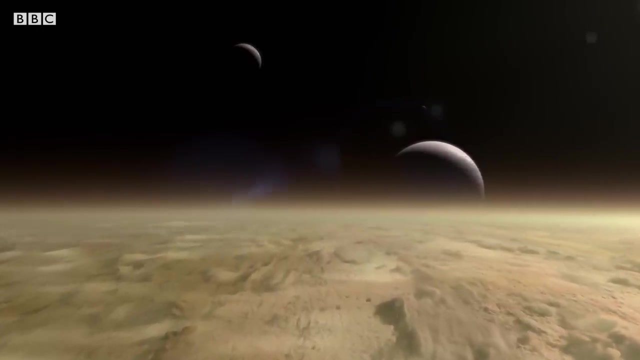 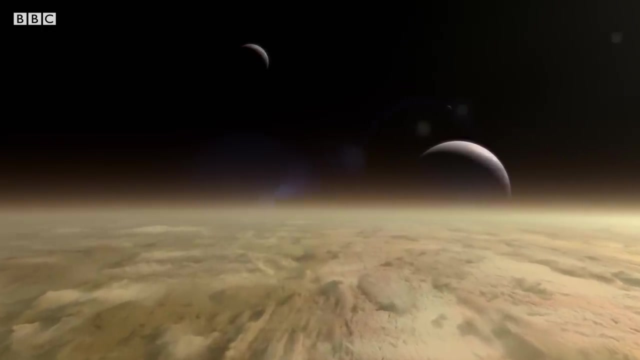 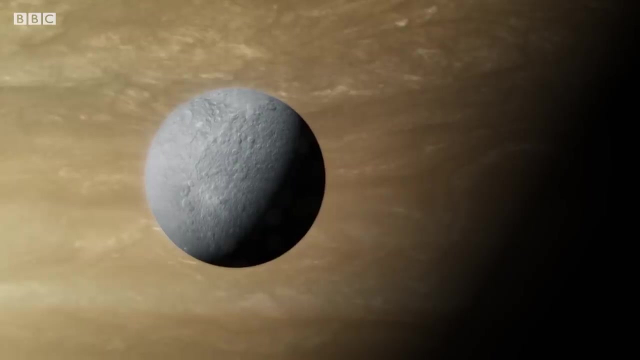 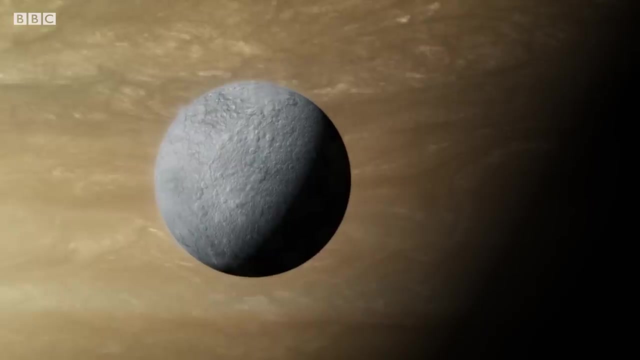 will literally rip you apart. You don't have enough gravity of your own to stay together. A leading theory suggests that, just beyond Saturn's atmosphere, an ice moon approaches close to or even just inside its Roche limit. As Saturn's immense gravitational force pulls it apart, the moon begins to rupture catastrophically. 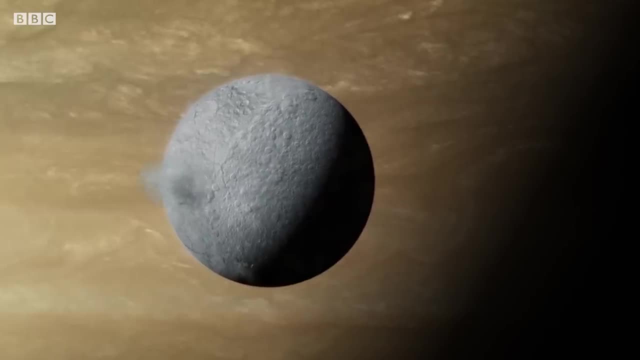 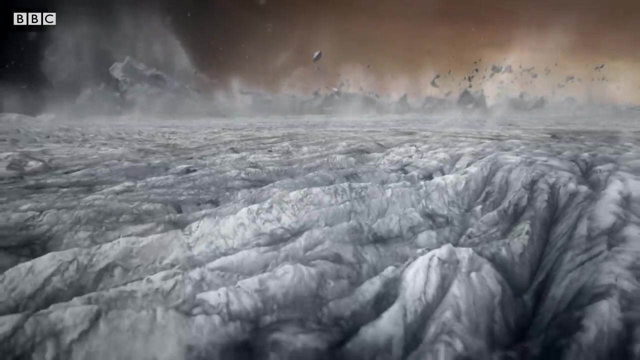 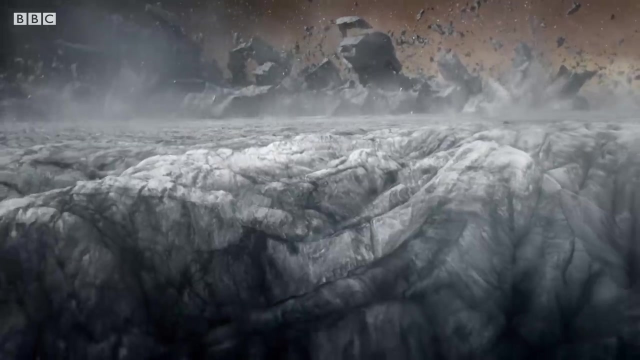 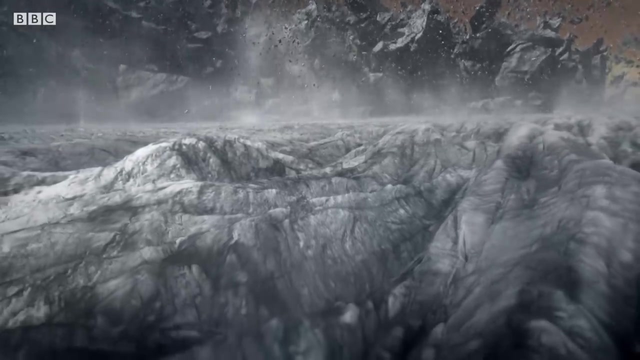 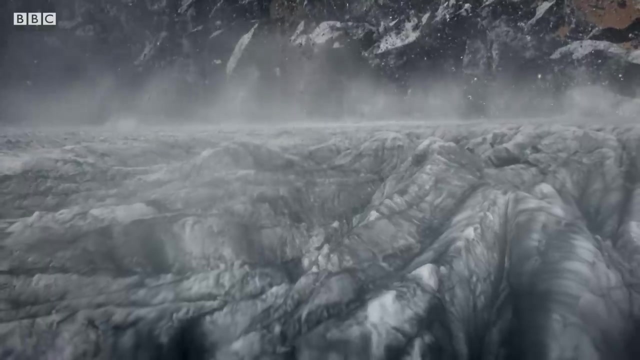 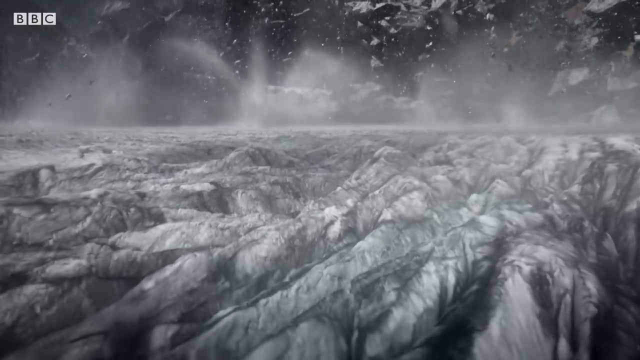 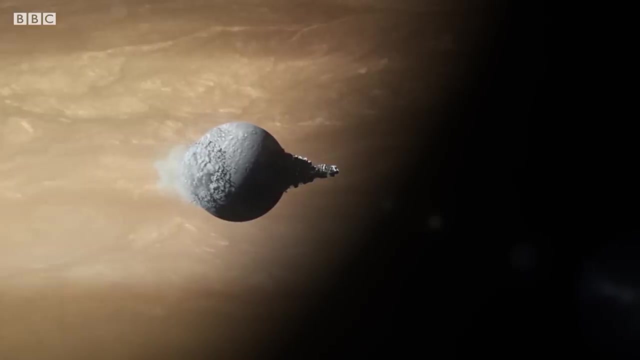 A world of ice, A world ripped apart by its proximity to a giant. Saturn soon falls into a new world, the Roche limit, where there are billions of ice masses that have been made available throughout the entire galaxy, Up to 17,000 trillion tons of ice. 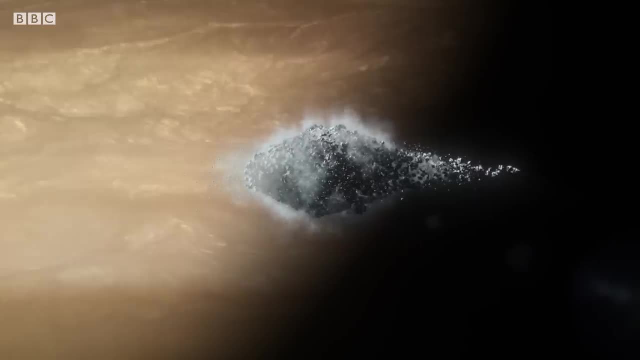 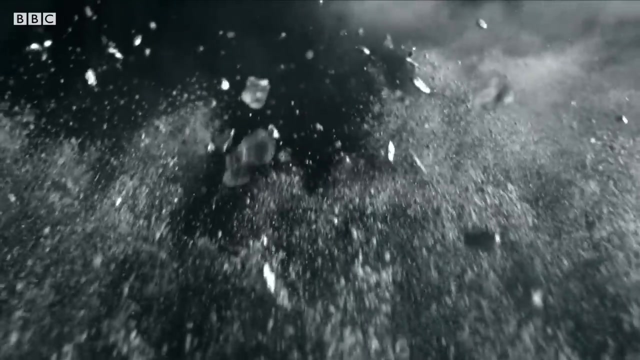 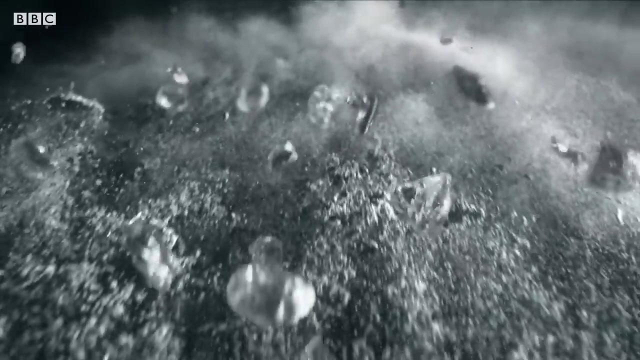 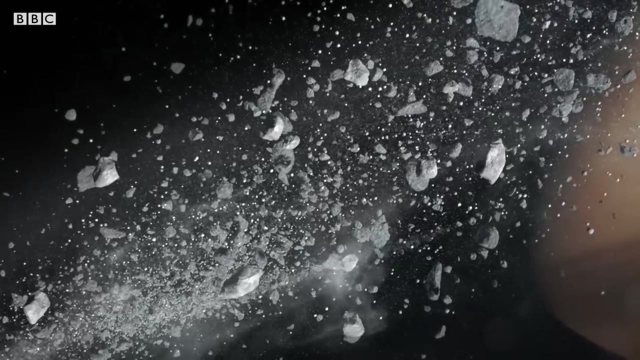 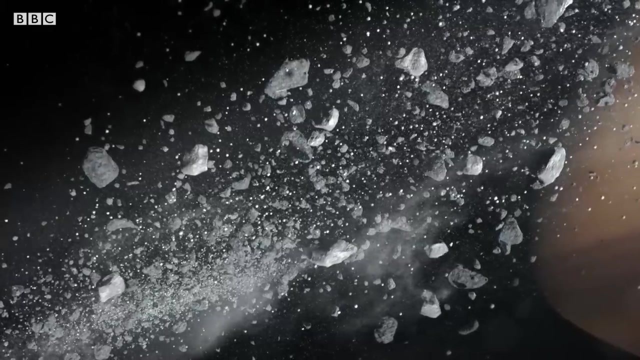 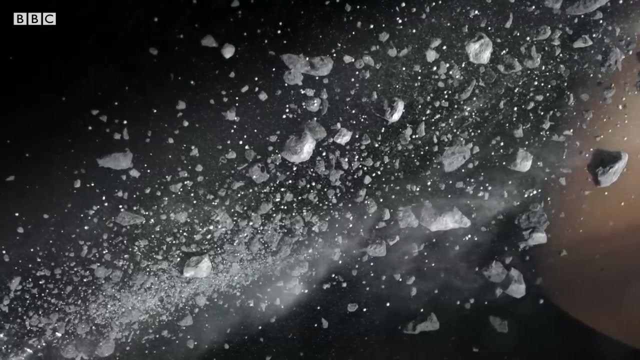 breaks apart in orbit of Saturn's star to the moon around Saturn, and thanks to the speeds this material is traveling, it's likely that in just a few days it spreads out to encircle the great giant. Saturn's iconic ring is now in place, but as Cassini turns its instruments towards it, it sees a single ring. 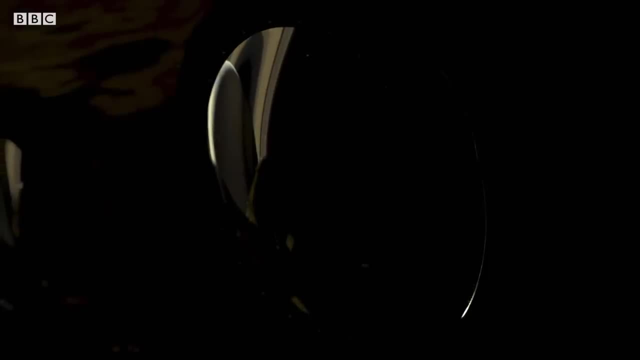 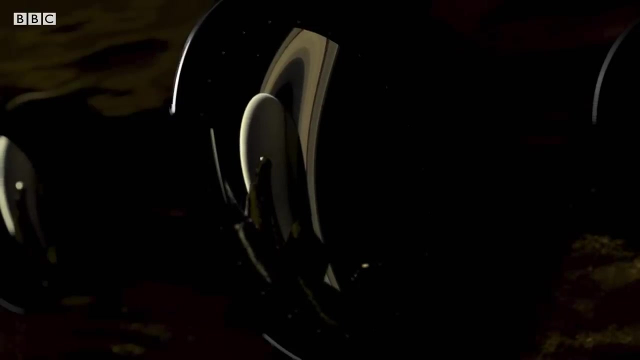 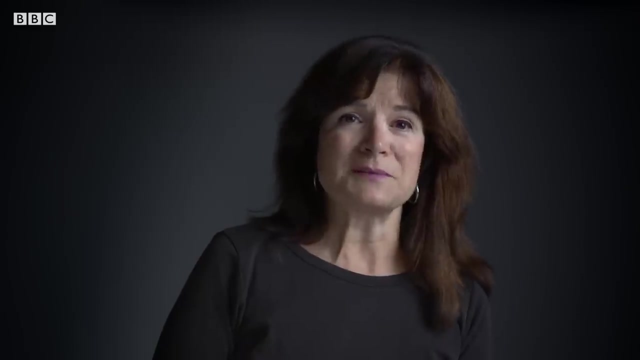 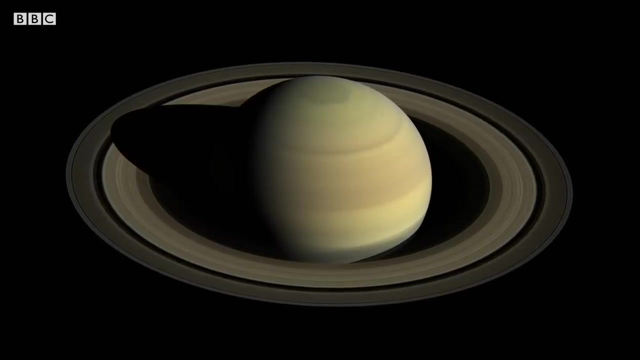 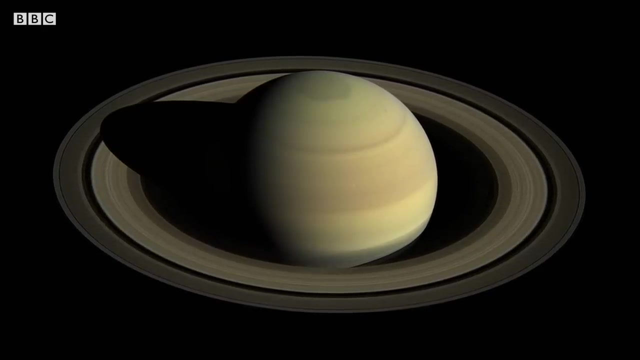 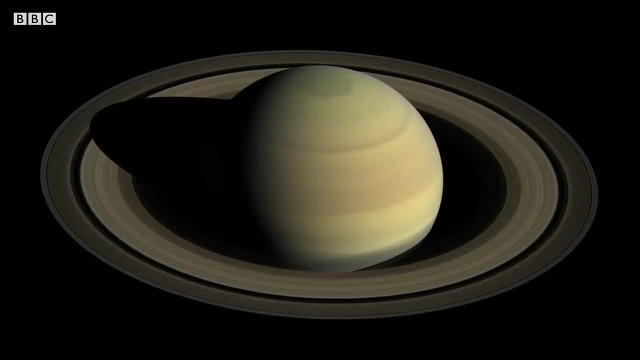 transformed the images we returned. they were phenomenal. they were resolution a factor of maybe 20 times better than anything we had had before. Cassini reveals how Saturn's giant rings have evolved. this debris now forms a disk wider than Jupiter, yet on average just 10 meters thick. 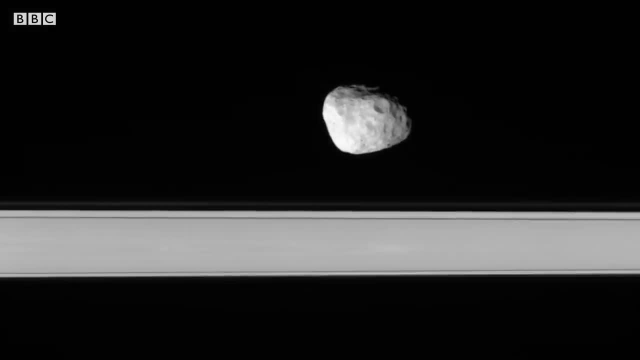 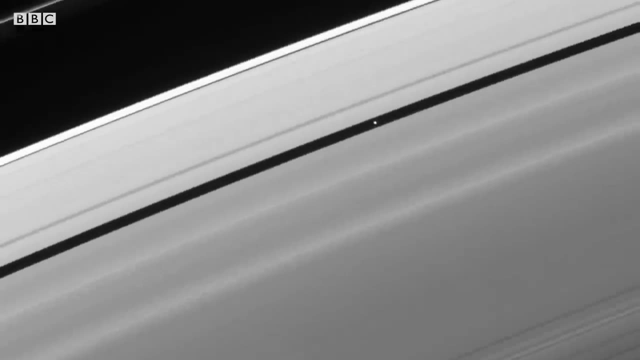 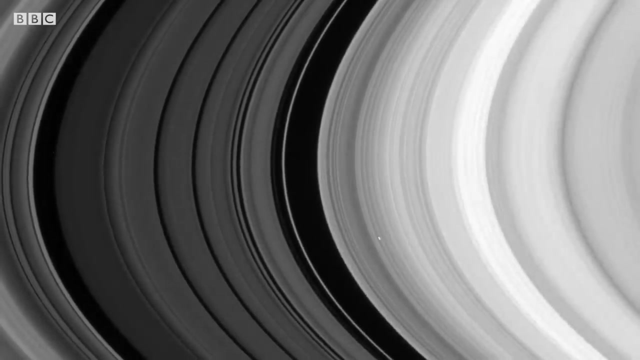 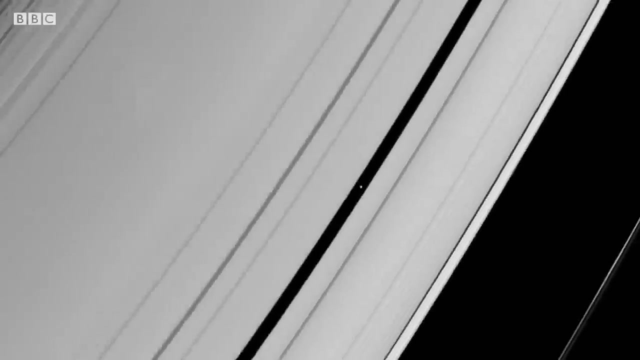 within moon sized chunks of ice orbit the structure, clearing great voids, turning one ring into many. but it's as Cassini captures images with the Sun directly above the equator that the most surprising feature of the Rings emerges. we knew this was going to be a 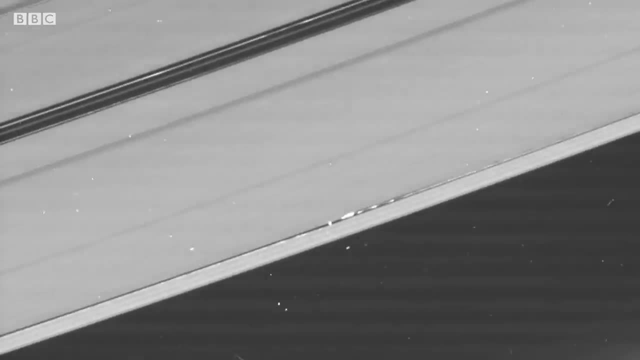 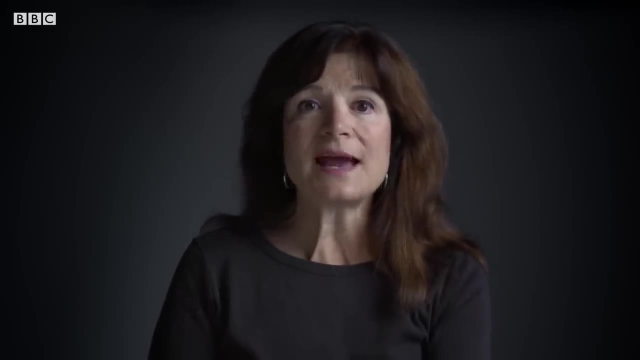 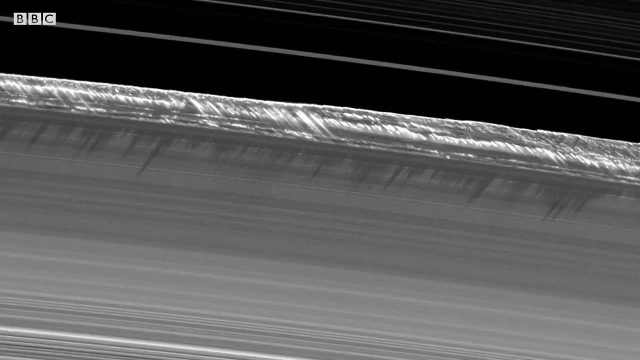 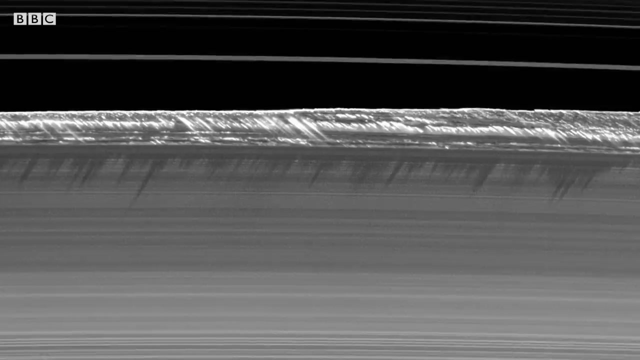 time for for us to investigate the third dimension, something that you don't get to see when you just look at picture of Saturn's rings, And what we found was staggering: Just right out of the gate we saw vertical structures. I just can't tell you how surprised we were to see this.